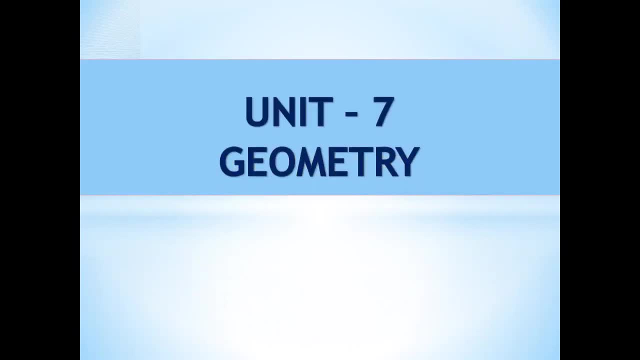 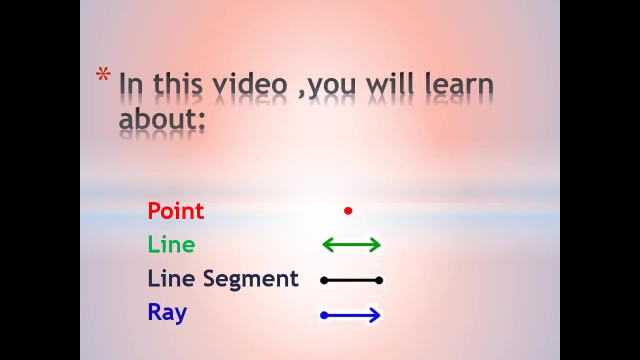 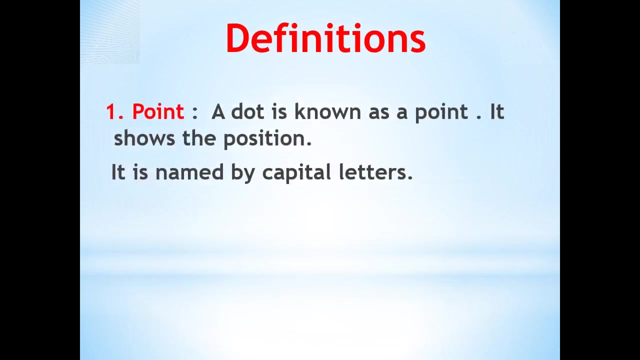 Hello children. today we are going to learn few geometrical concepts. In this video you will learn about point, line, line, segment and array. First of all, let us learn what is a point. A dot is known as a point. It shows us the position. We name points by capital letter, For example. here we are having the points. 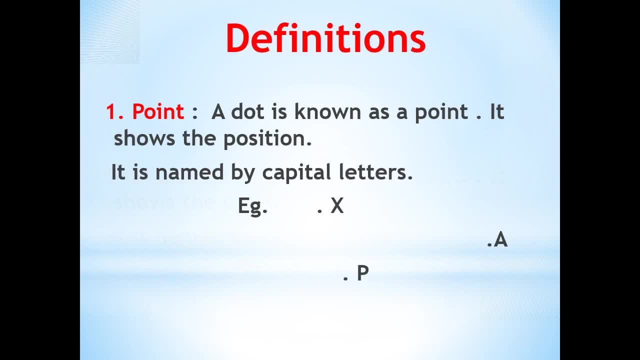 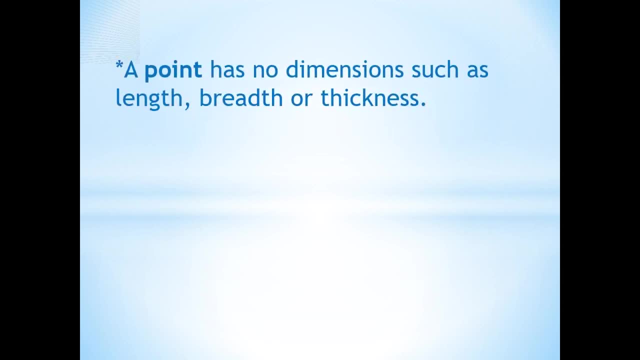 point x, point a and point p. A point has no dimensions, That is, it has no length, no breadth and no thickness. Few examples of points are the sharpened end of a pencil, the pointed end of a needle. Now, if we have a look on this map, we come to know that 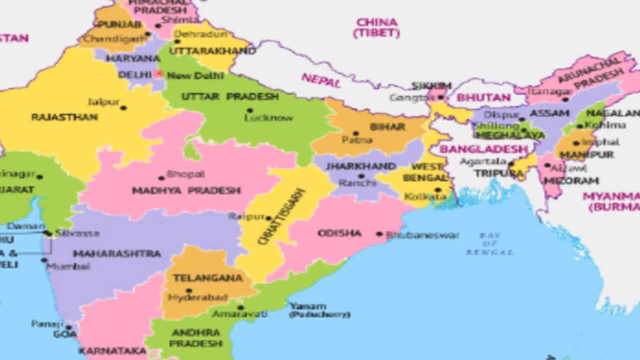 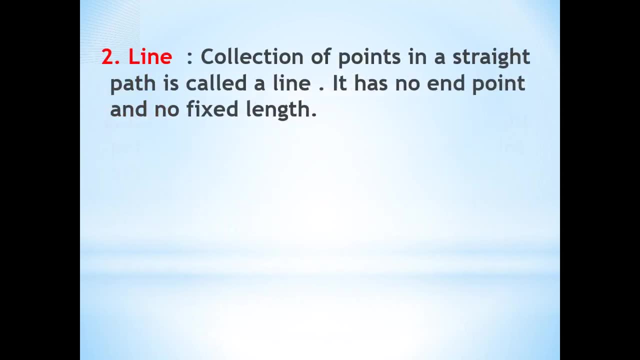 we use point to locate states and their capitals. Now let us learn about line. A collection of points in a straight path is called a line. A line has no end point and no fixed length. Here we are having the line ab. This line ab has no beginning and no ending. 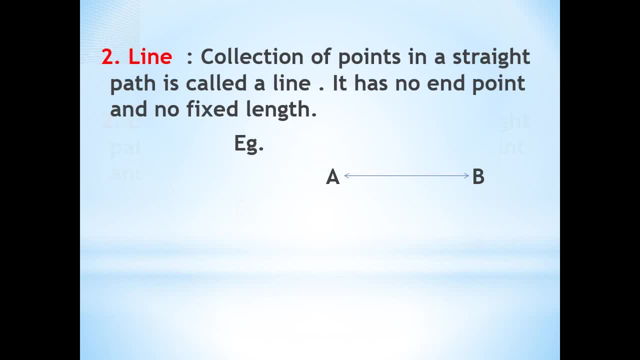 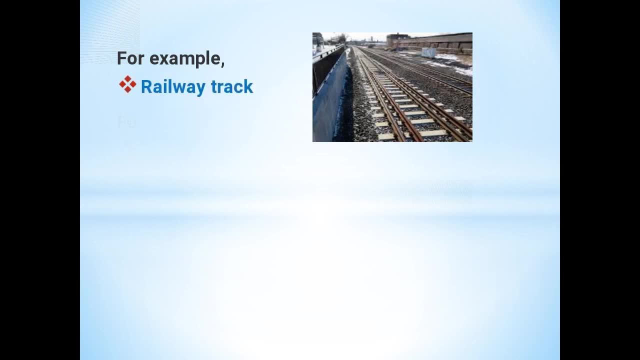 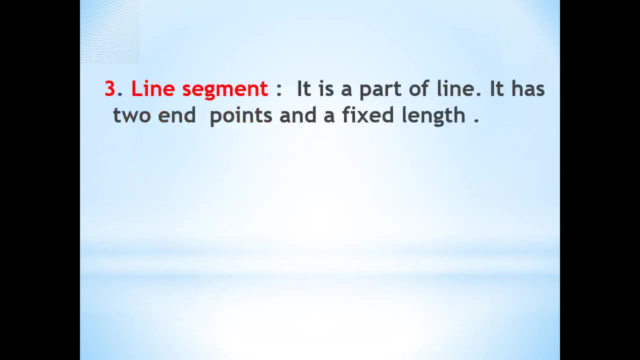 Furthermore, we cannot measure the length of this line. Few examples of line are railway track, road and orbit of the planets. Now let us learn about line segment. A line segment is a part of a line. It has two end points. that is, one starting point and one ending point. 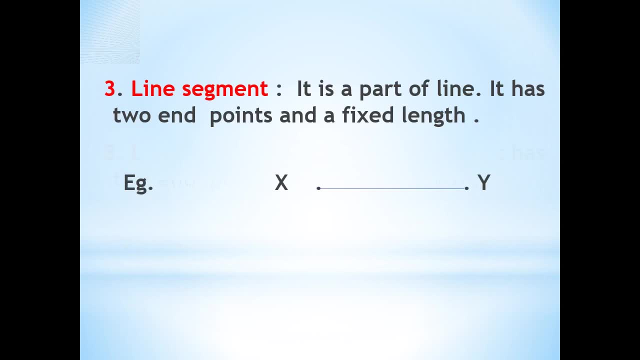 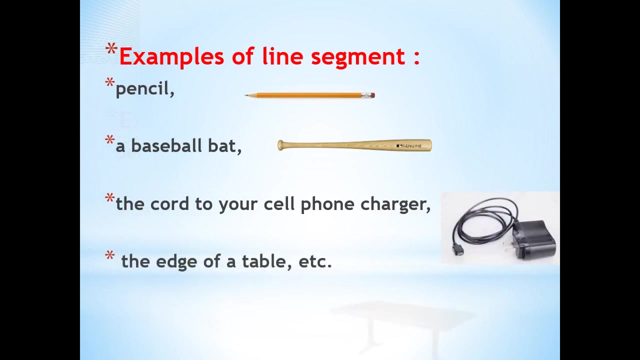 it has a fixed length. for example, XY is a line segment. it is having one starting point and one end point and we can use a ruler to find the length of this line segment. now, few examples of line segments are pencil, baseball bat, the quad to your cell phone charger and the edge of a table. let us learn about ray. 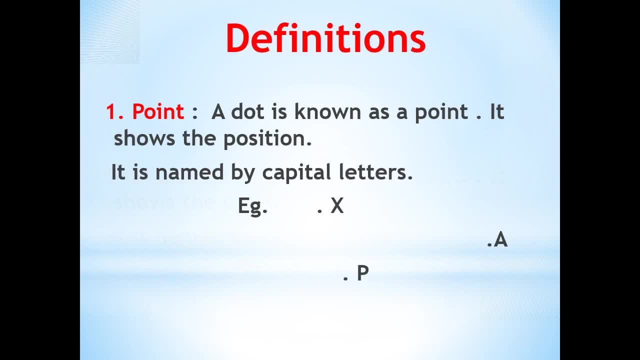 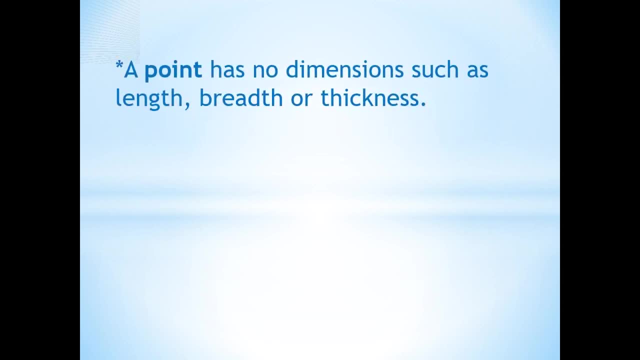 point x, point a and point p. A point has no dimensions, That is, it has no length, no breadth and no thickness. Few examples of points are the sharpened end of a pencil, the pointed end of a needle. Now, if we have a look on this map, we come to know that 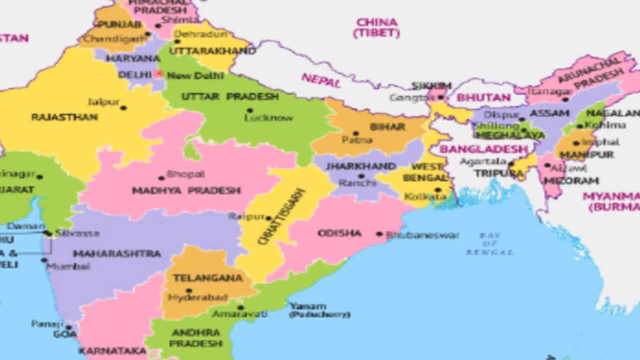 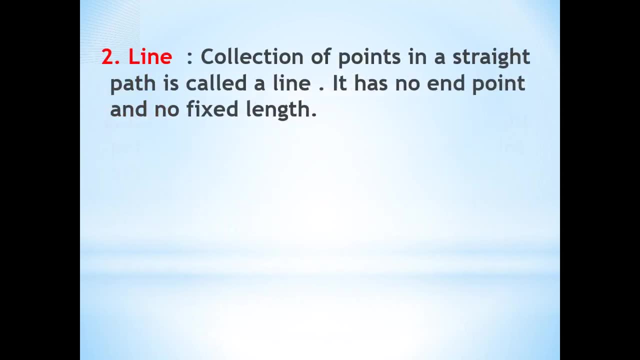 we use point to locate states and their capitals. Now let us learn about line. A collection of points in a straight path is called a line. A line has no end point and no fixed length. Here we are having the line ab. This line ab has no beginning and no ending. 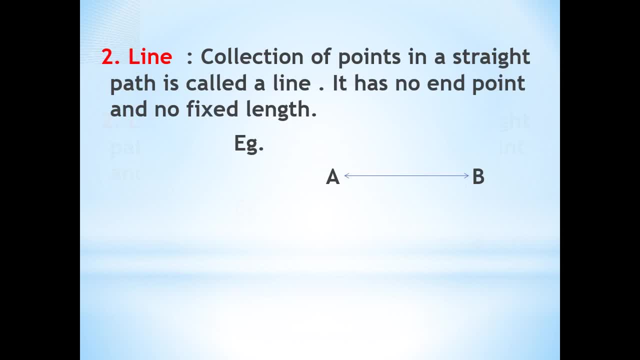 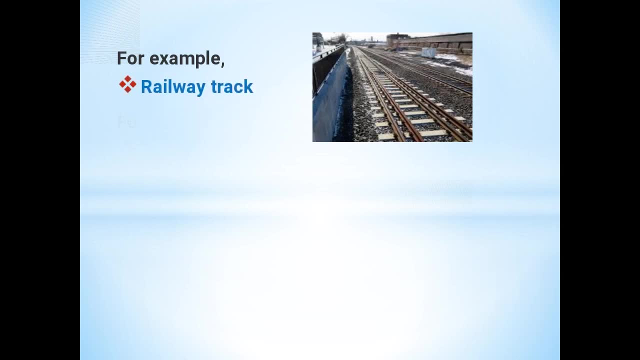 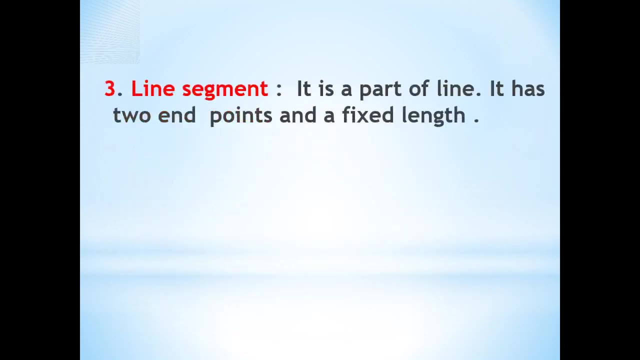 Furthermore, we cannot measure the length of this line. Few examples of line are railway track, road and orbit of the planets. now let us learn about line segment. A line segment is a part of a line. It has two end points. that is one starting point. 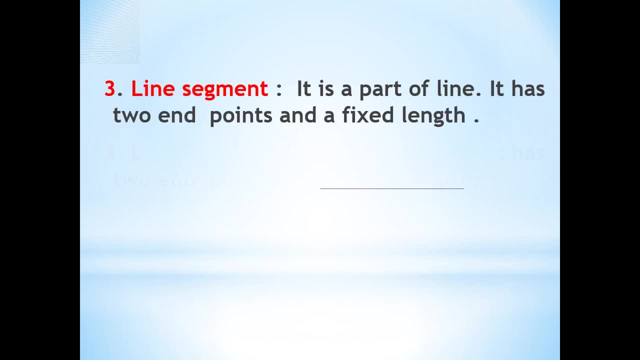 and one ending point and it has a fixed length. for example, XY is a line segment. it is having one starting point and one end point and we can use a ruler to find the length of this line segment. now, few examples of line segments are pencil, baseball bat, the. 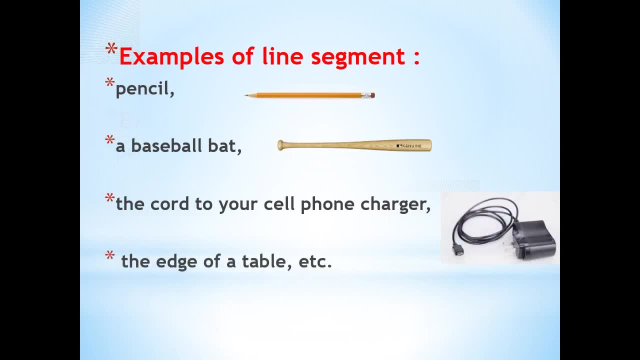 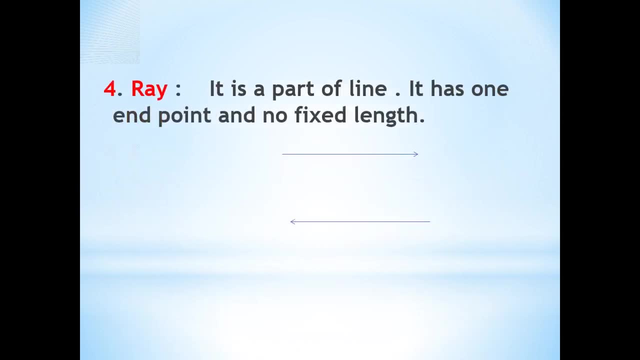 cord to your cell phone charger and the edge of a table. let us learn about ray. ray is also the part of line. it has one end point and no fixed length. we are having the two rays here. one is a ray OP, another is the ray BA. ray OP has the